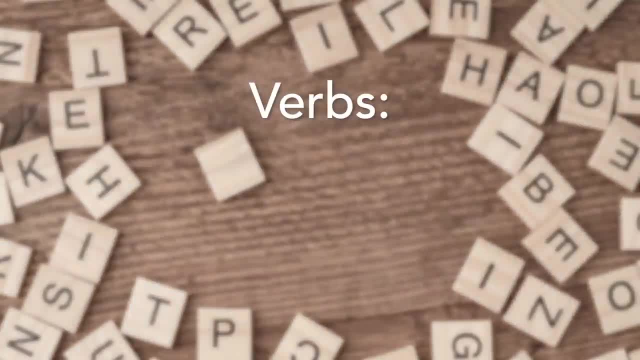 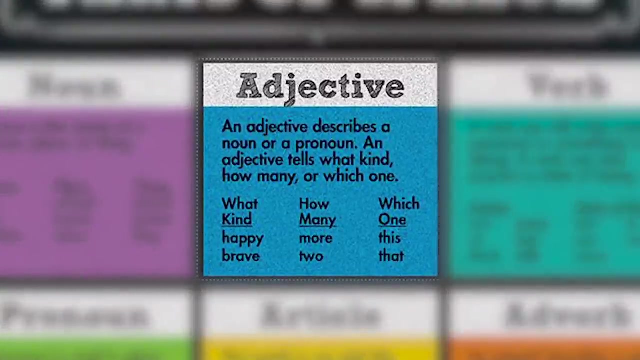 nouns like boy or dog or house. You've got your verbs like run, play or dance, And you've got your adjectives like smart or curious, As we mentioned above. obviously, not all words are adjectives, only special ones. We use adjectives in sentences to describe what a noun is like. 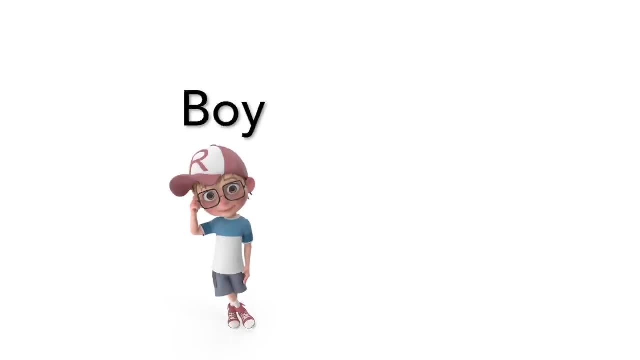 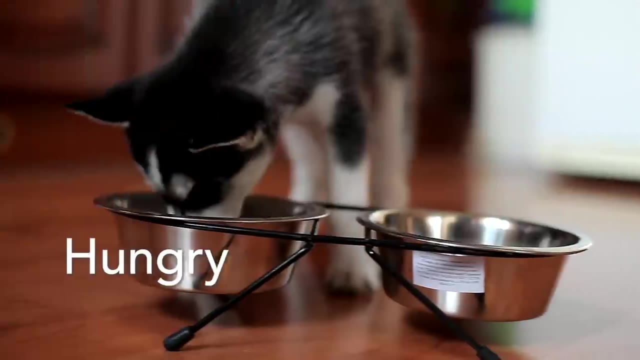 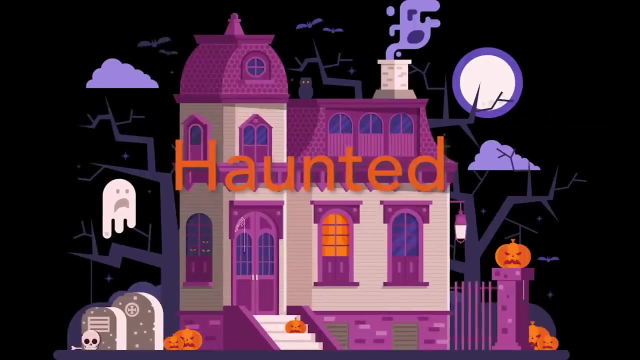 or to give it characteristics. So instead of just boy we could say tall boy, The adjective there is tall. Or instead of the dog, we could say hungry dog, with hungry as our adjective. Instead of a dog we could say a dog, And then we're done. So why do we use adjectives? Well, without. 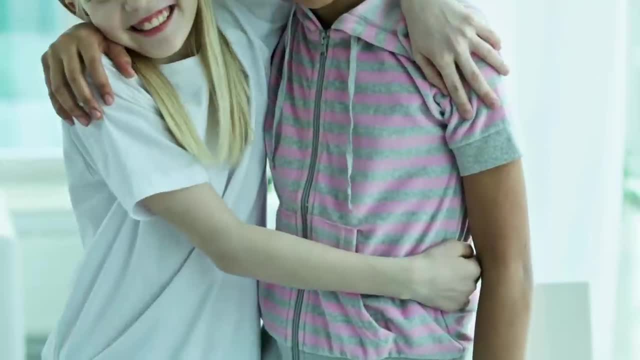 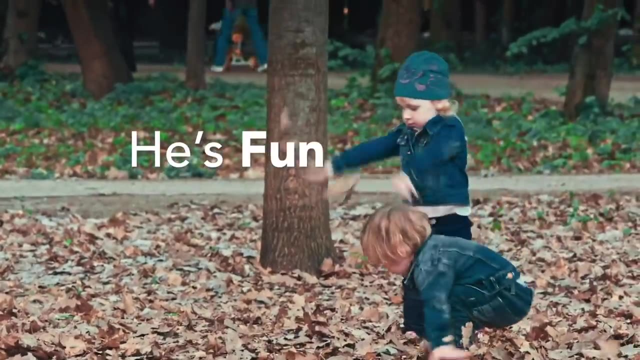 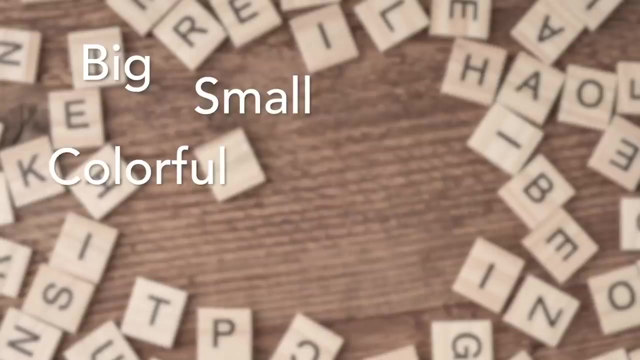 them, we wouldn't be able to describe what things are like. If someone asks you what your best friend is like, you'd need an adjective to describe him or her, As in he's fun or she's athletic, He's cool or she's intelligent. Adjectives are our way of telling other people what the things around us. 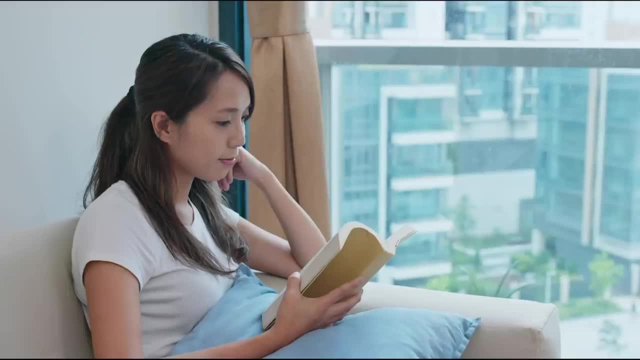 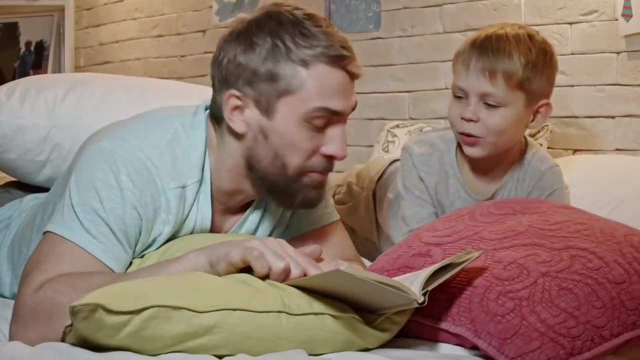 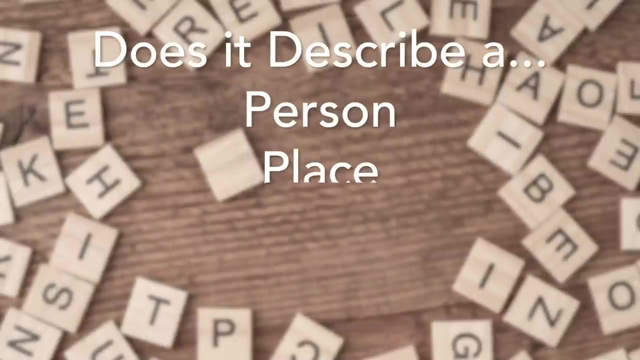 and characteristics are and how we think of them. So how do you know if a word is an adjective when you're reading or listening to a book or a story? Here's a simple test to check if a word is an adjective, Ask yourself this: Does it describe a person, place, thing or idea? Does it give you? 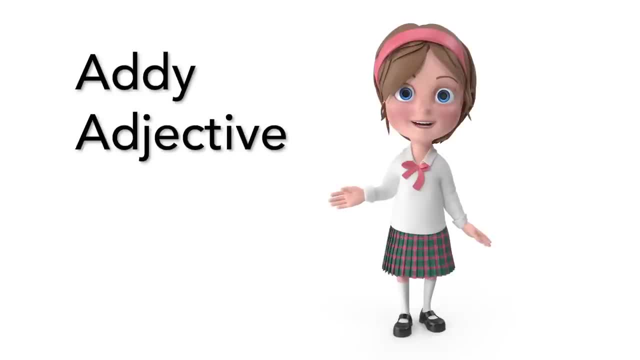 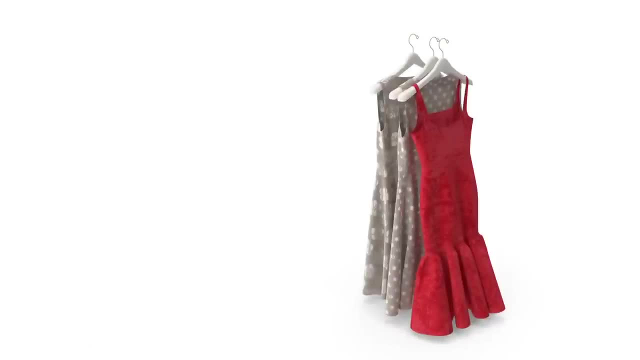 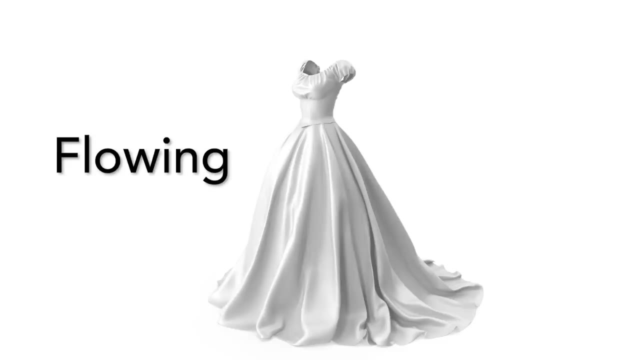 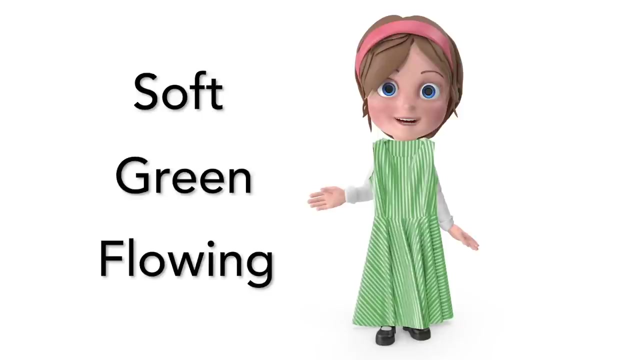 a detail about a noun. This is Addie Adjective. Her job is to add information to nouns. For example, imagine Addie is wearing a dress. The word dress is a noun. What's the dress like? Is it green, flowing, flowery, sparkly, soft? Let's say: Addie is wearing a soft, green, flowing dress. 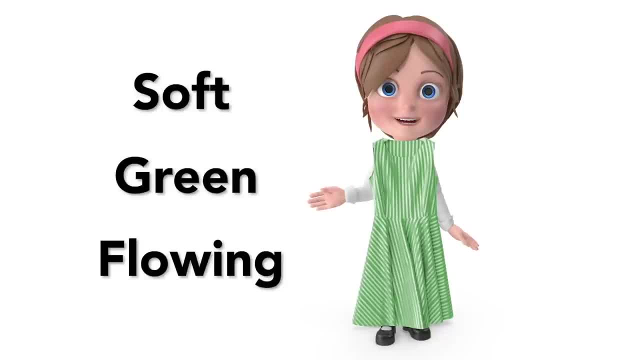 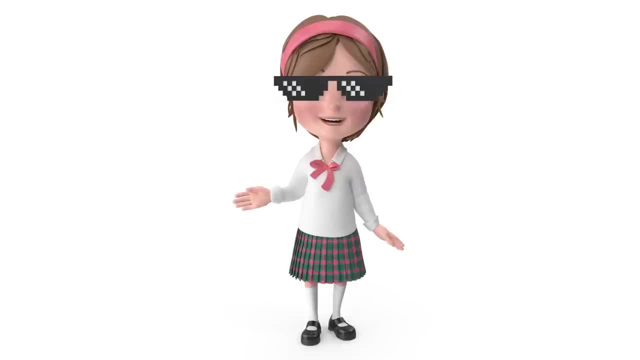 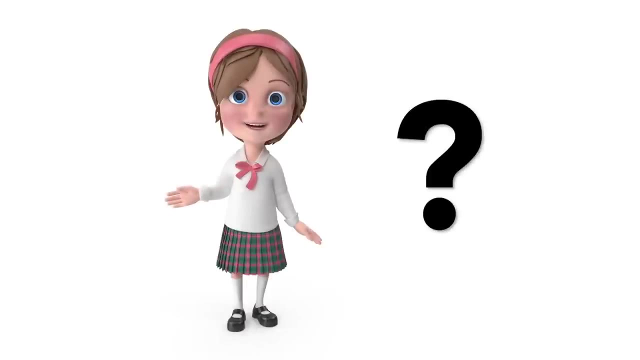 In that sentence. soft, green and flowing are all the adjectives. Now Addie is wearing glasses. What are those glasses like? We need adjectives to tell us. Are they round, square, blue, dark? What else is Addie like? Every word we use to describe her is an adjective. Is she?